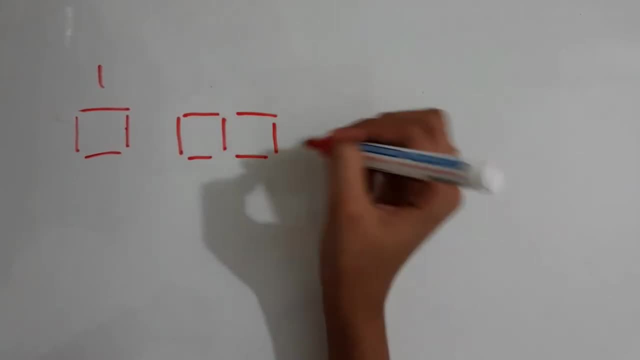 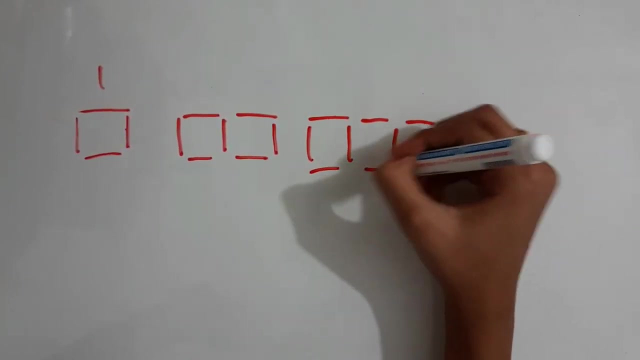 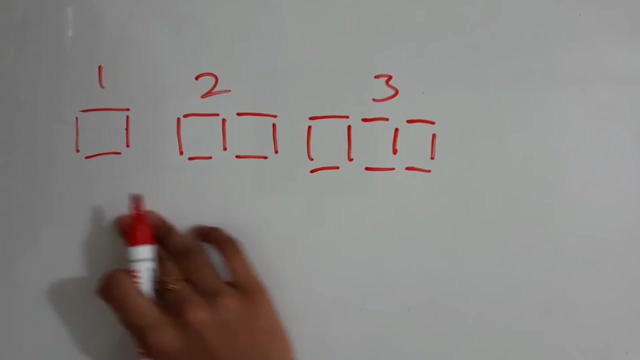 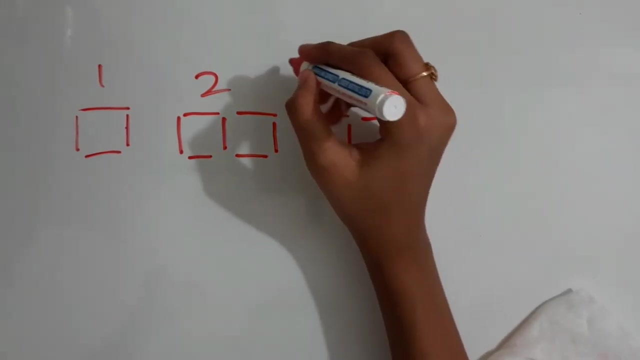 second one, the second figure, like it keeps on following, this is the second figure and this is the third figure. so we can do this, we can go on to 50,000 and 10,000, but it's very difficult if you get a question like: what is the 50th figure of this, of this figure? so, 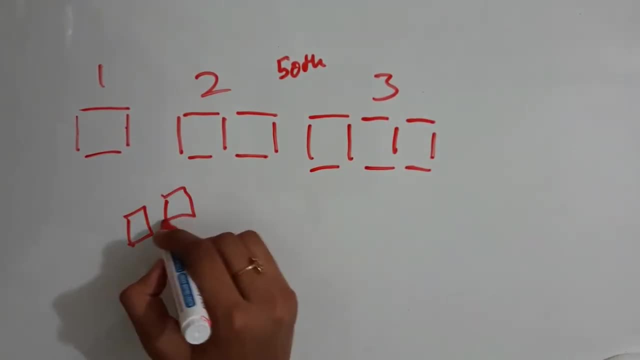 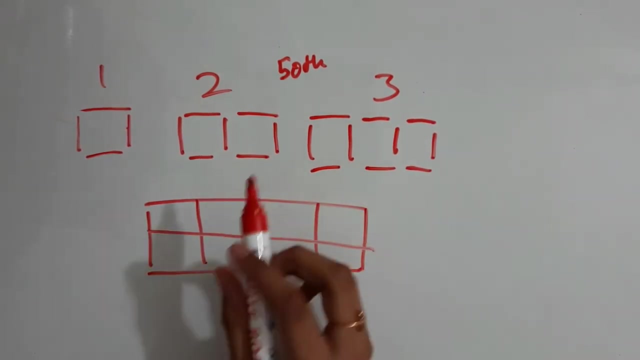 you can't keep drawing boxes like till 50, so there's a trick over here: just put: I'll just draw another box over here and divide it into four, and I'm gonna write N. N stands for number and M stands for matchstick. the first figure has four matchsticks: one, two, three, four, four matchsticks, the: 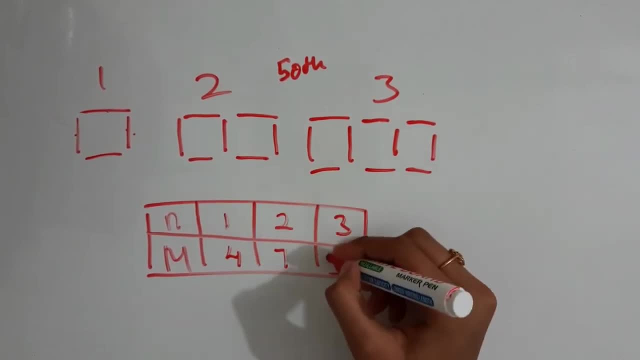 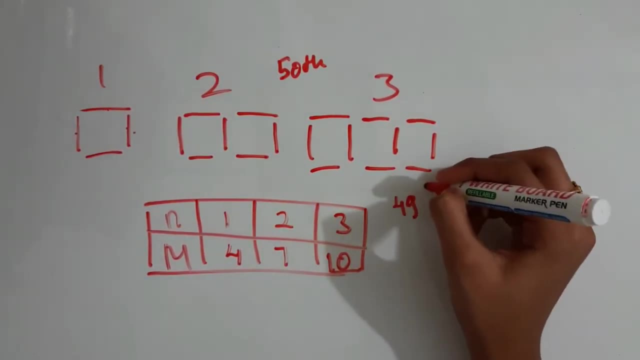 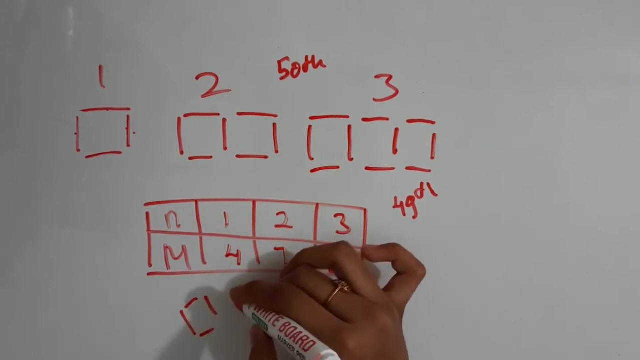 second figure has seven and the third figure has tenth. so if you get a question like for find the matchsticks for the 49th figure, you can't keep drawing boxes like one, two and like that. that's insane. so the formula is: so we should see that how many mattress ifs are increasing for 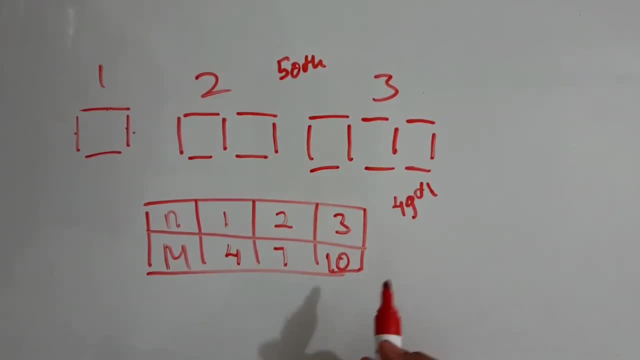 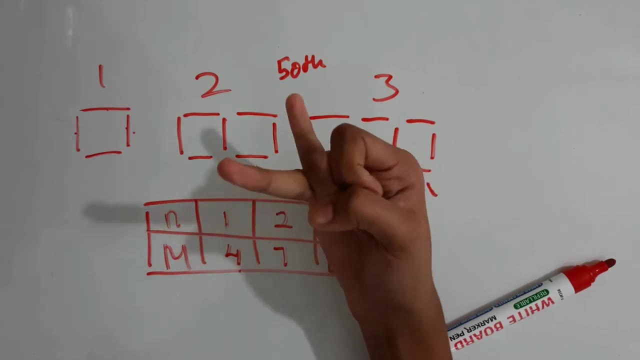 each figure. so over here it was 4 and the second was 7, 4, 5, 6, 7, so it's increasing by 3, 1, 2, 3, so I want 10, 7, 8, 9, 10, it's increasing, and then 8, 9, 10. 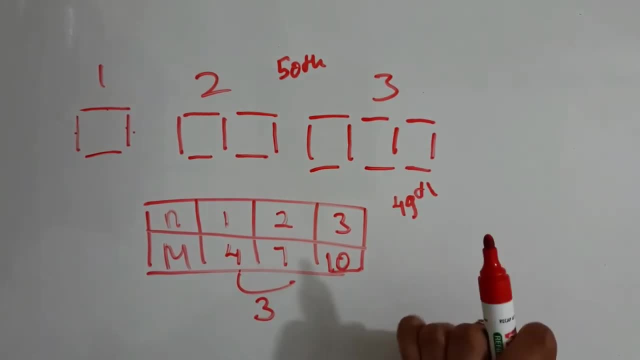 but it's increasing. and if you changed the formula twice or three times, you got that the formula was 7, 9, 8, 10, so lots of more numbers. did you al possible think about that? but I tried to figure it out. this one for one method. 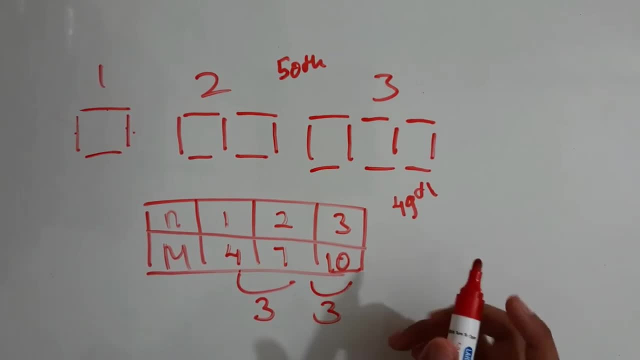 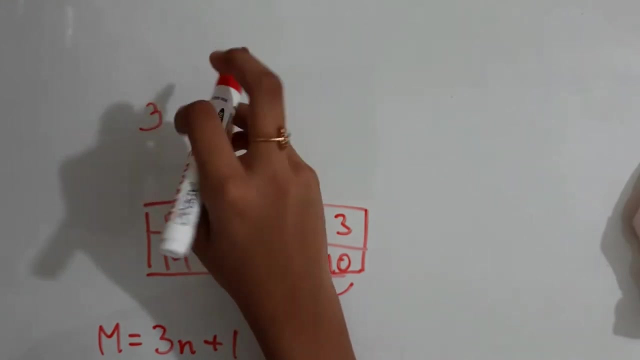 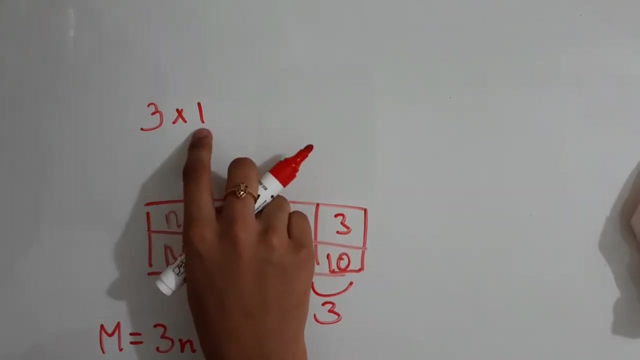 it's increasing by 3 over here. so the formula is: M equals 3, n plus 1. so let's check it out with the formula: okay, 3 into 1, because over here n the first one is one. so I am multiplying it by 1 plus 1 plus 1 equals 3 into 1. 3 plus 1 equals 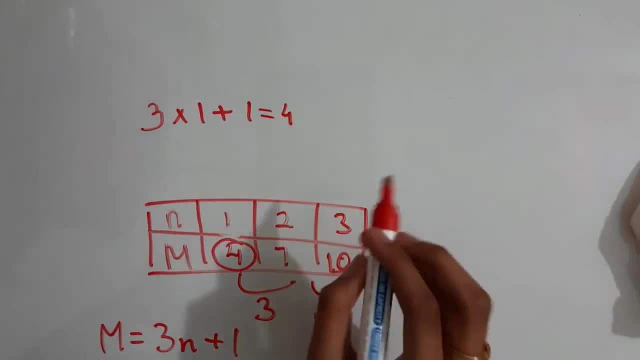 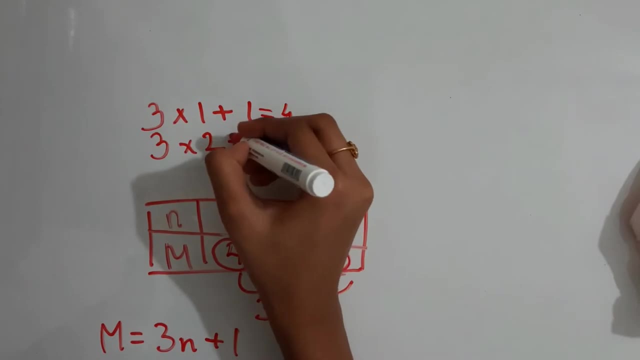 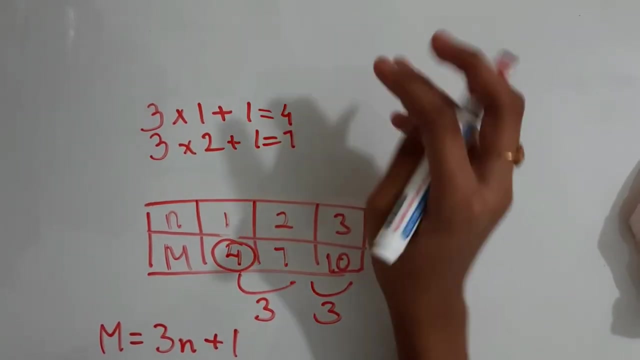 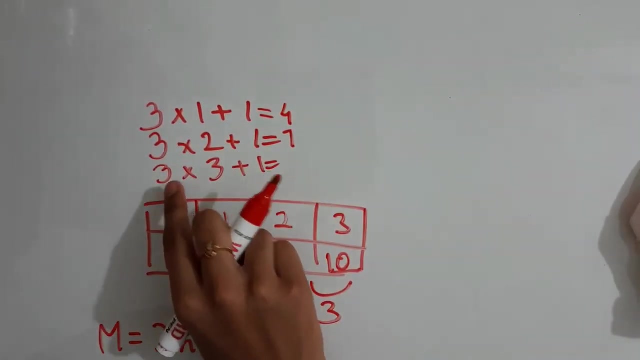 4, so we got the first figures matchsticks. so let's try the second: 3 into 2 plus 1 equals 3 into 2, 6 plus 1: 7. we got it. so the third one: 3 into 3 plus 1 equals 3 into 3, 9, 9 plus 1: 10. so we got it correctly. so we have. 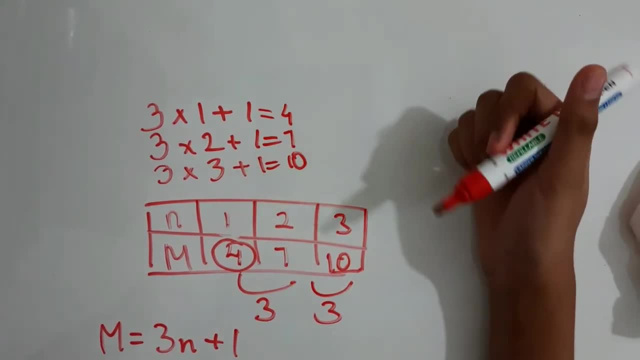 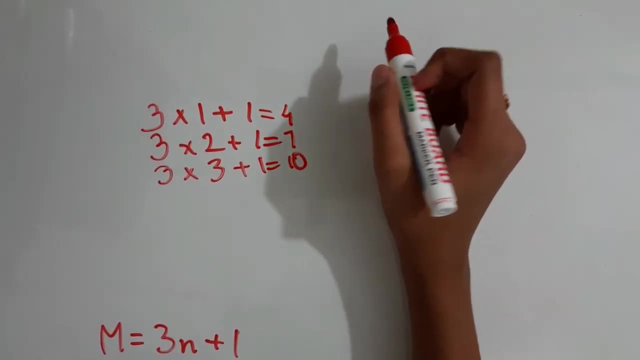 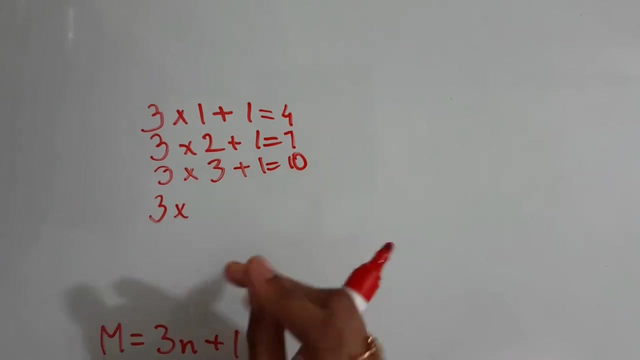 confidence that we might get the bigger numbers correctly. so suppose you get a question like: find the 50th figure, so because it's increasing by 3, we should write 3 into its 58th right. so 3 into 50 plus 1, 3 into 50 equals 150, 150 plus 1. 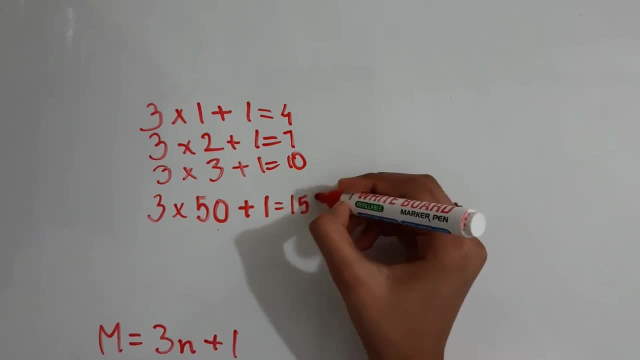 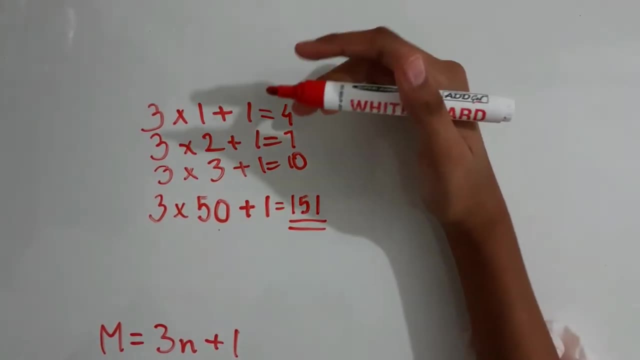 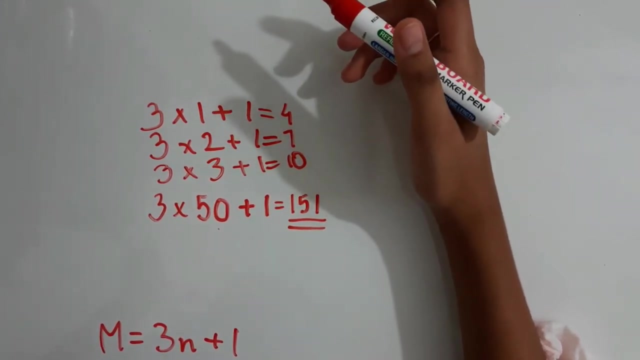 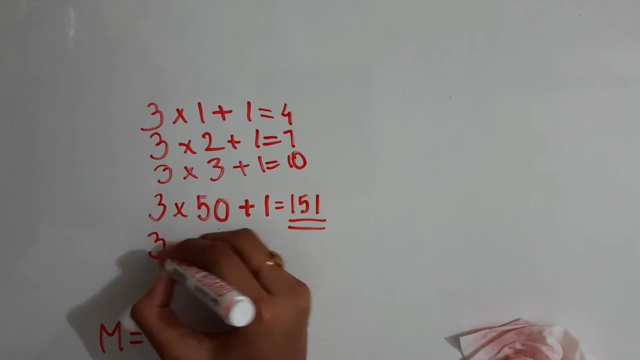 equals 151, so the answer is 151. so the 50th figure has 151 matchsticks. so we we can take another example, for instance the 12th figure 3 into 12. you'd always write the formula first plus 1. 12th figure 3 into 12. we should. 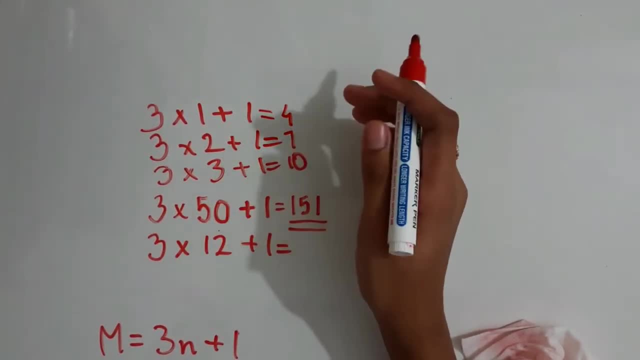 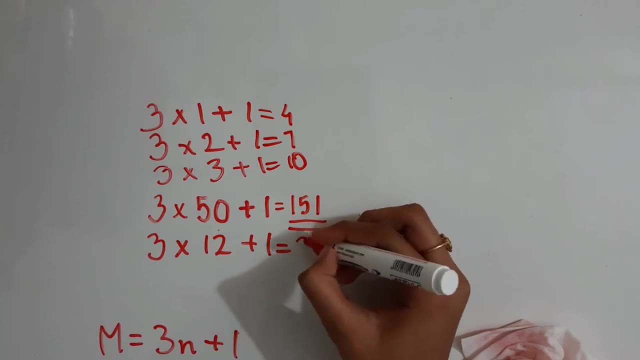 find out how many match sticks are there in that twelfth figure. so 3 into 12 is 36, 36 plus 1 is 37. So there are 37 mastics in the 12th figure. You can check it out. 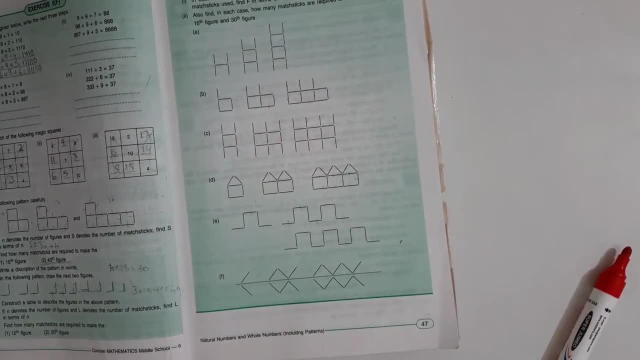 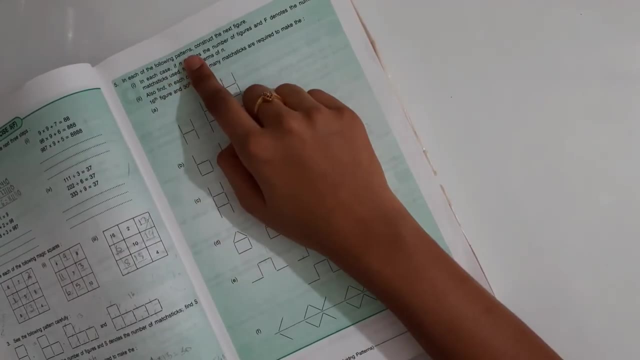 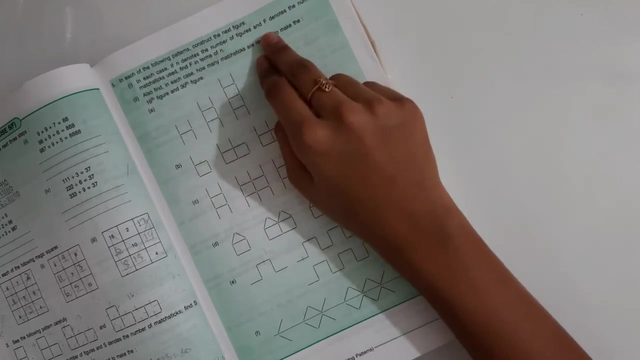 It's correct, So I'm going to give you more examples. So let's take the first one in the book. In each of the following patterns, construct the next figure In each case. if n denotes the number of figures and f denotes the number of mastics used, find f in terms of n. 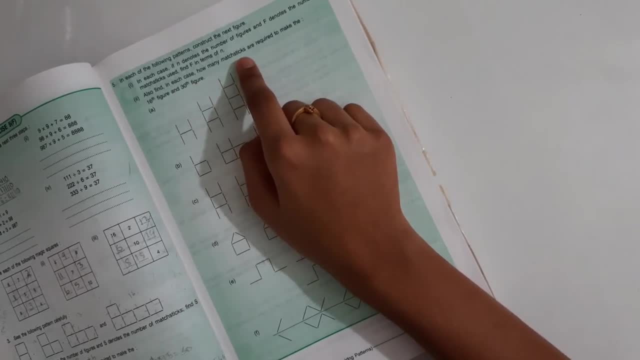 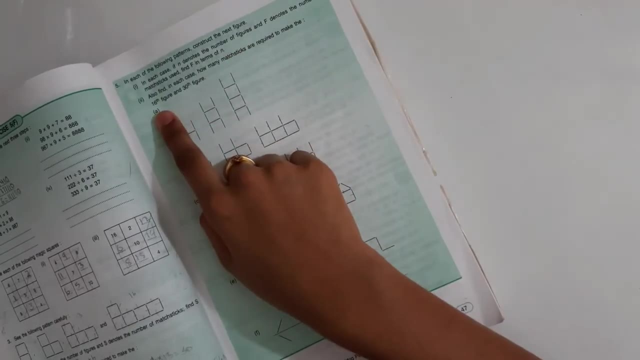 Also find in each case how many mastics are required to make the 16th and the 30th figure. We should find how many mastics are used for the 16th and the 30th. So the first one is this: 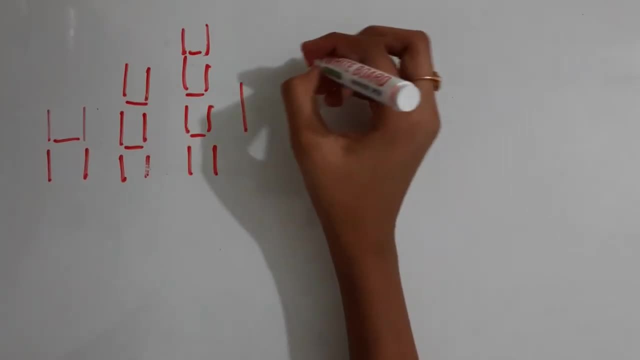 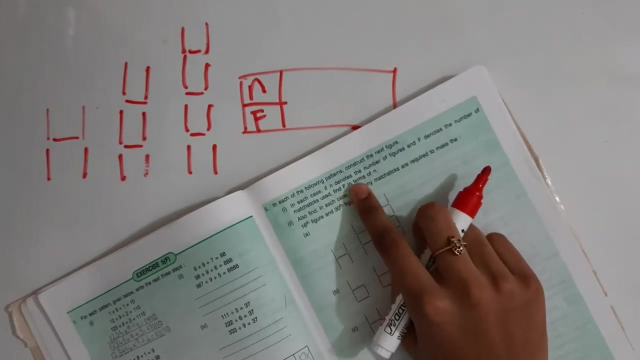 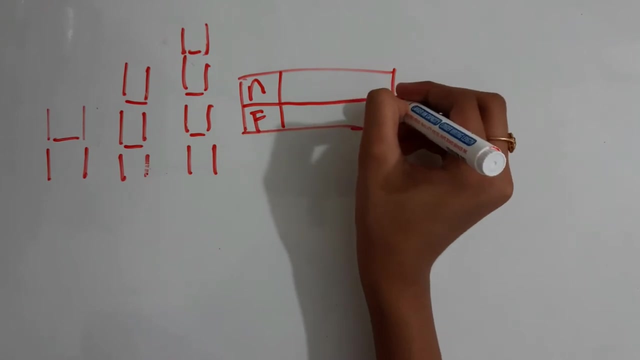 So let's start. So, as I told, draw a box, So we'll keep n and f. They said that find f in terms of n, So I'm writing f instead of m. So the first figure. 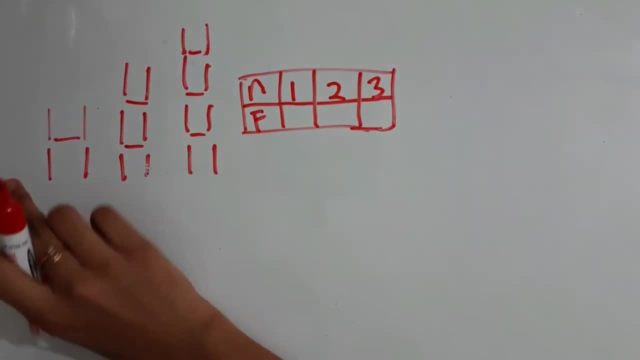 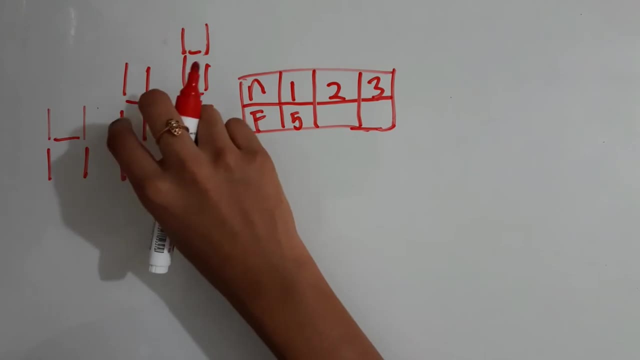 The second, The third, The second one and the third one. The first one has 1,, 2,, 3,, 4,, 5. 5.. 1, 2,, 3,, 4,, 5,, 6,, 7, 8.. 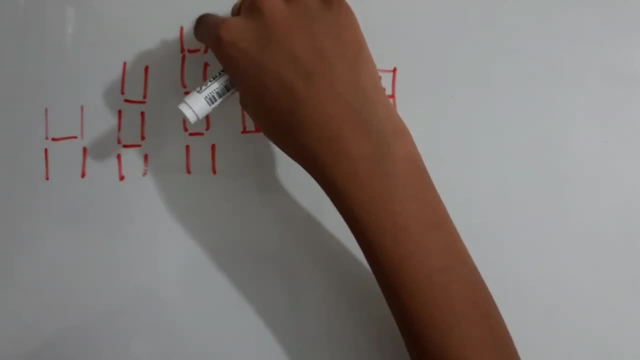 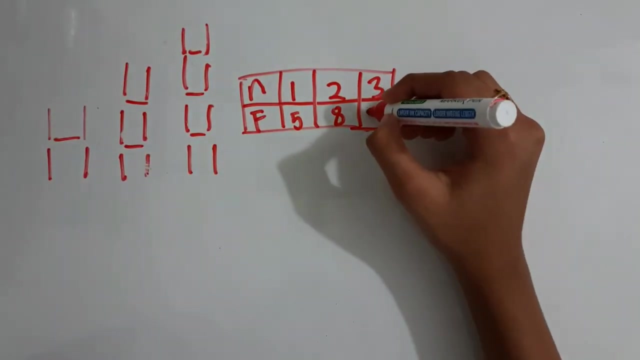 The second figure has 8.. 1,, 2,, 3,, 4,, 5,, 6,, 7,, 8,, 9,, 10,, 11. 11.. The third one has 11 mastics. 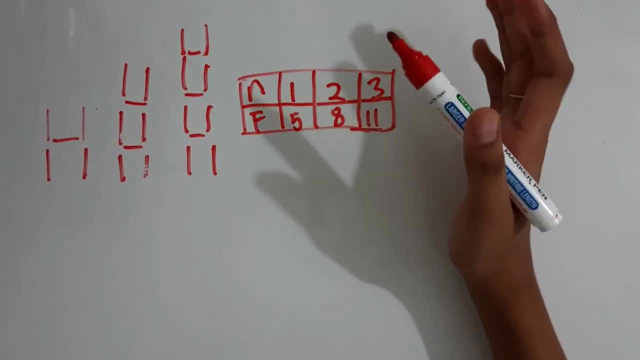 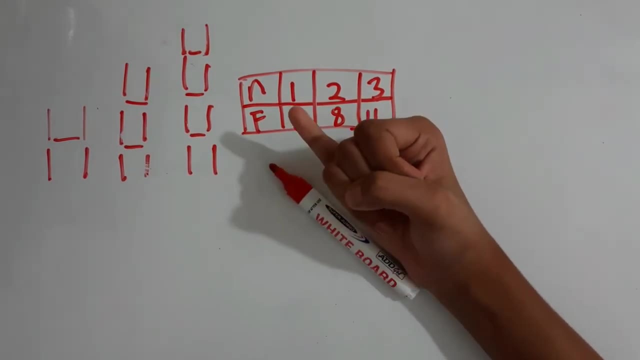 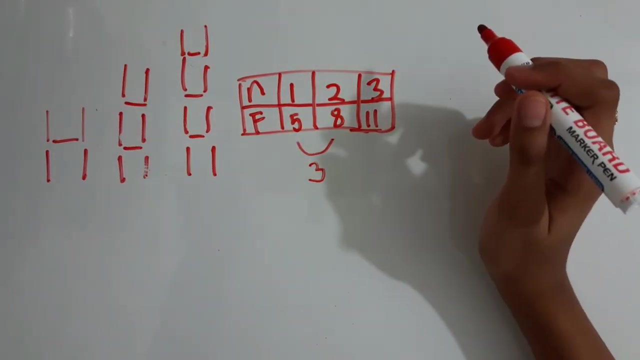 Now we are going to See how many mastics are increasing. So 5 and 8. 5,, 6,, 7,, 8. 3. So 3,, 9,, 10,, 11.. 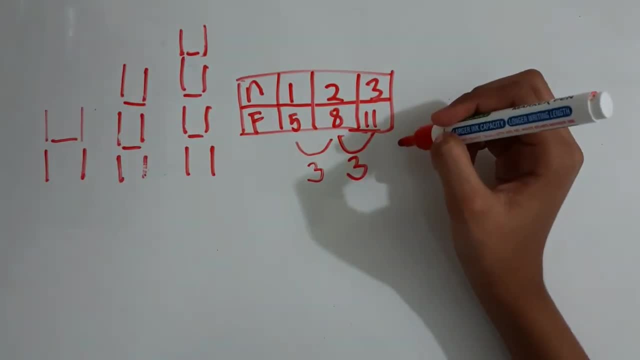 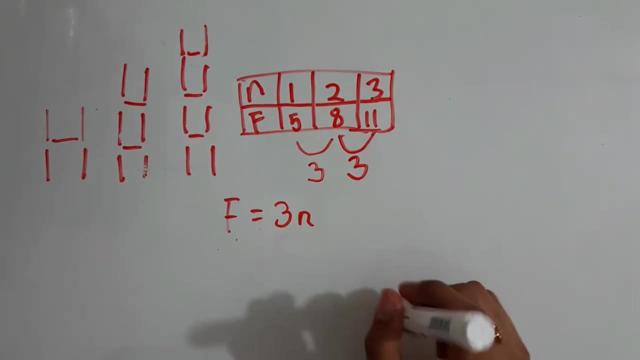 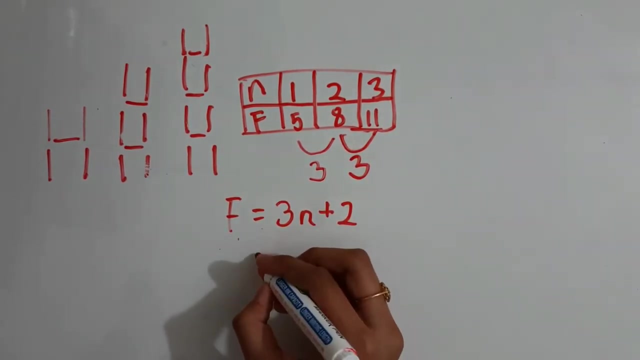 3. So we hear 3. Our formula is: f equals 3n Plus 2.. So let's check the formula. So 3 into 1 plus 2 equals. We are going to check for the first figure. 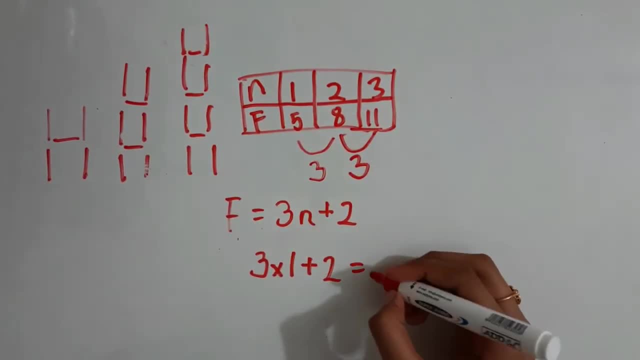 3 into 1 equals 3.. 3 plus 2 equals 5.. So the first figure has 5 mastics. So let's check it for 2.. 3 into 2 equals 6.. 6 plus 2 equals 6.. 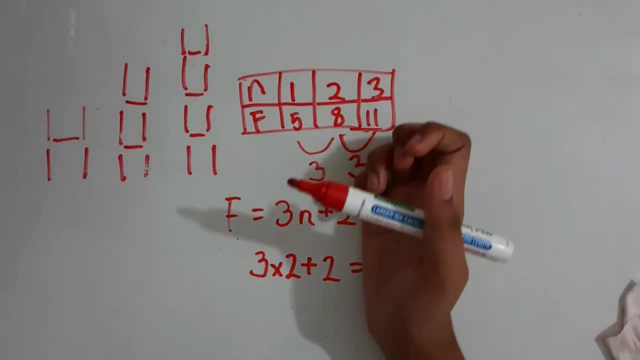 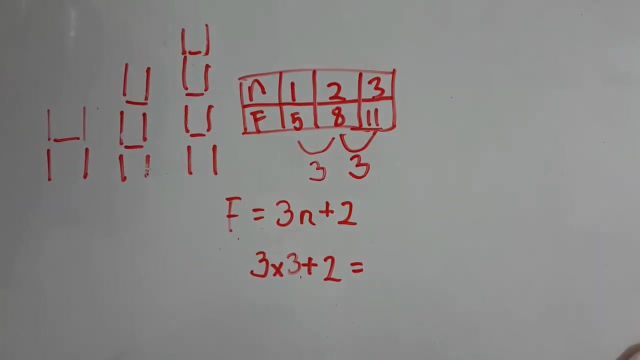 6 plus 2 equals 8.. So we got it. So let's check for third figure: 3.. 3 into 3. Plus 2. 3 into 3 equals 9.. Plus 2 equals 9 and plus 2 equals 11.. 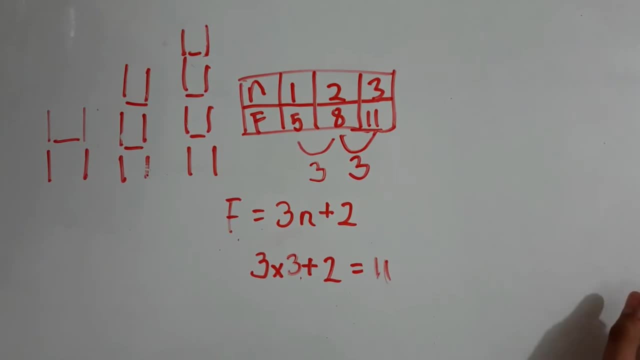 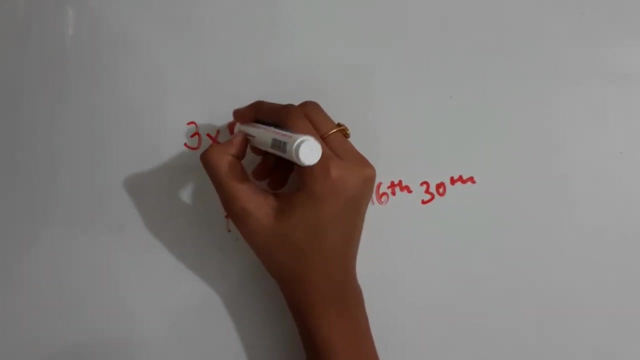 So we got it. So now we can check for the sixteenth figure. So now we can check for the sixteenth figure and 38th figure. so now we got our formula here. so 3 into 16 plus 2, 3, 16s. 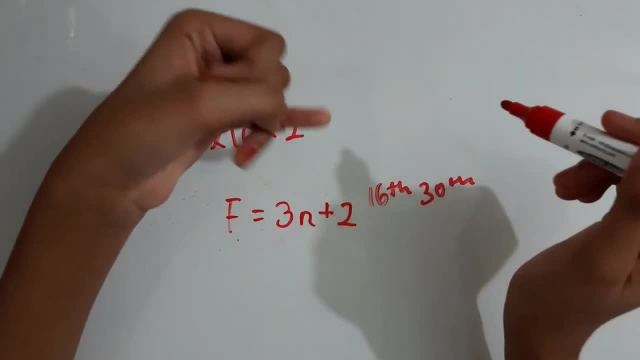 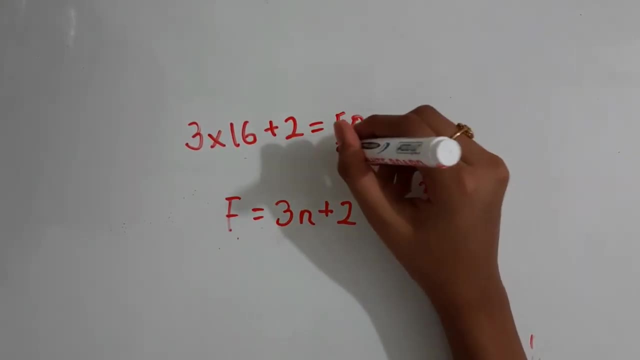 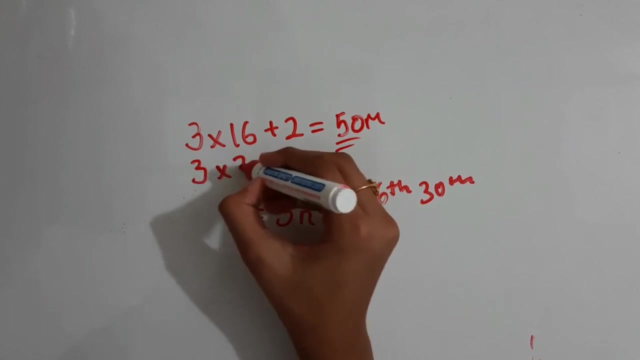 are 48, 48 plus 2, 49, 50. so the number of matchsticks used in the 16 figure is 50 matchsticks. so now let's find for the 38th: 3 into 30 plus 2, 3 into 30 equals. 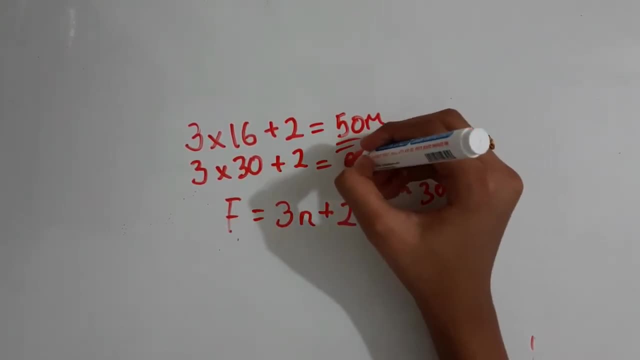 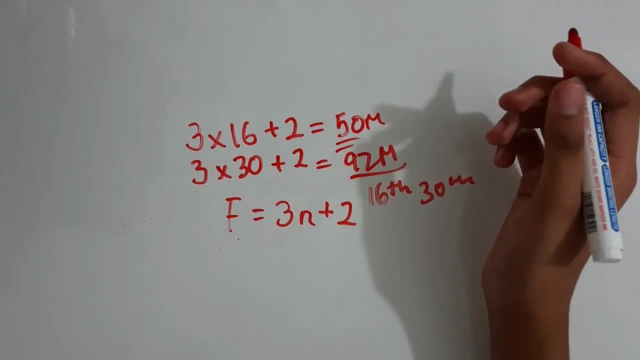 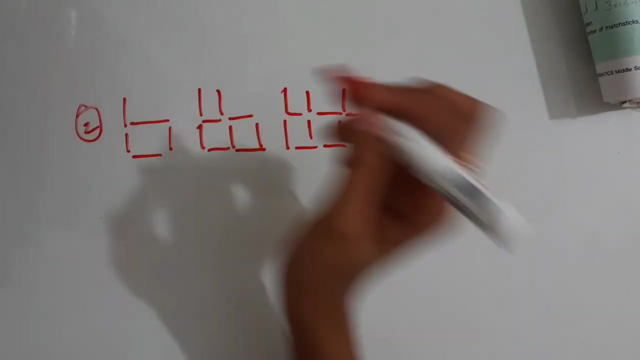 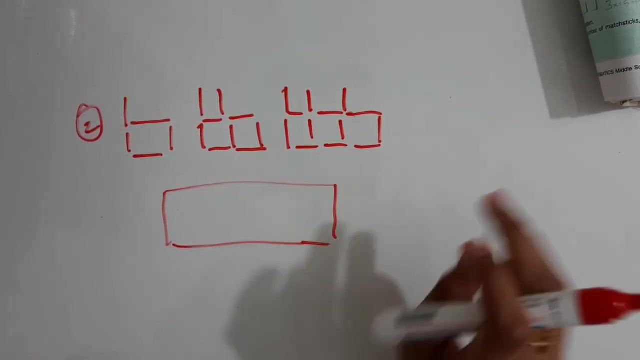 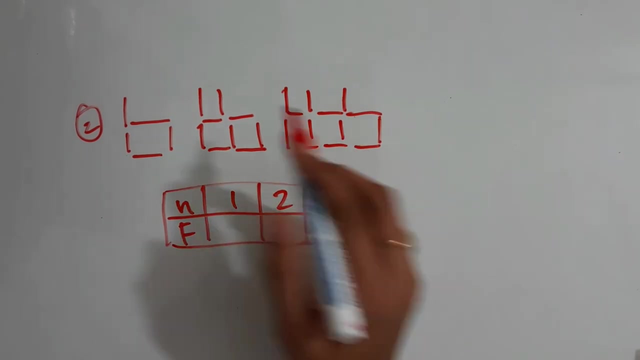 90, 90 plus 2 equals 92 matchsticks. so in the 38th figure there will be 92 matchsticks. so we finished the first one. let's check on the second question. so let's draw a box, divide it: N and F: 1, 2, 3, 1, 2, 3, 4, 5. the first figure has 5, 1, 2. 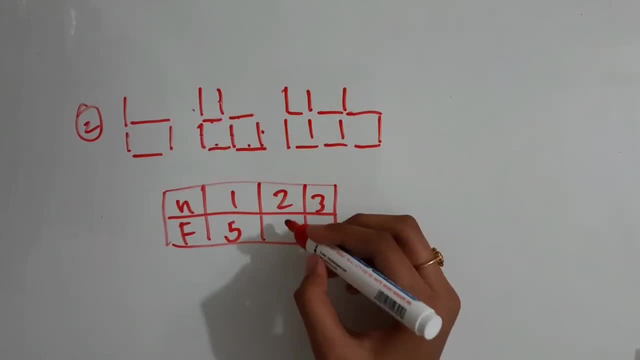 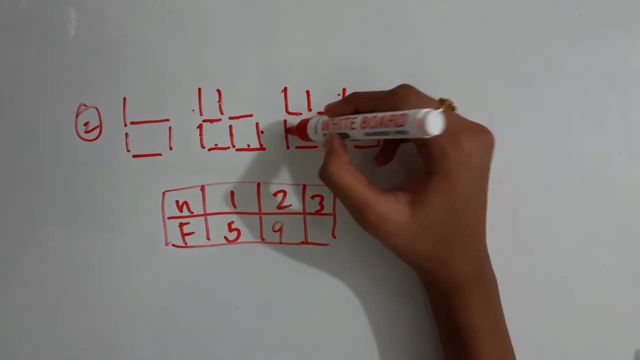 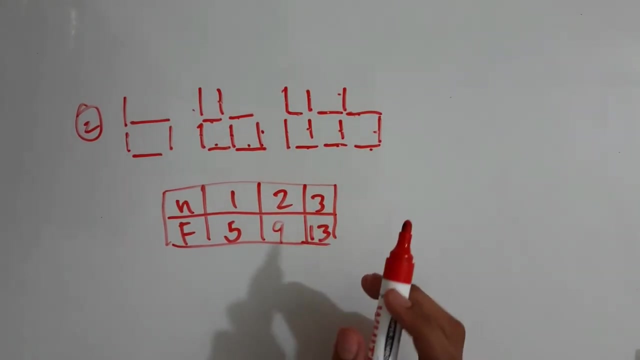 3, 4, 5, 6, 7, 8, 9. the second figure has 9 matchsticks and third figure has 1, 2, 3, 4, 5, 6, 7, 8, 9, 10, 11, 12, 13, 13 matchsticks. so let's see how, by how much it increases the first one. 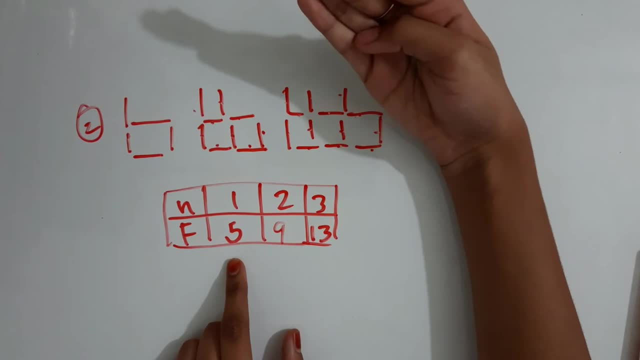 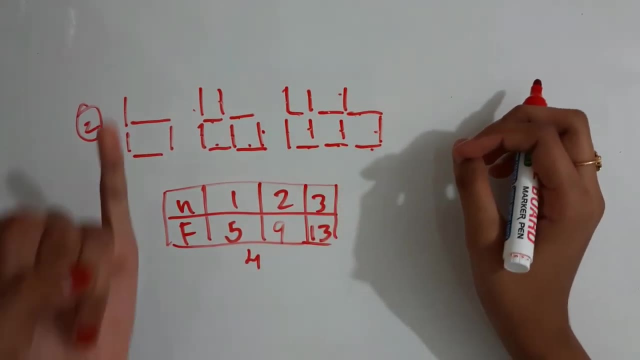 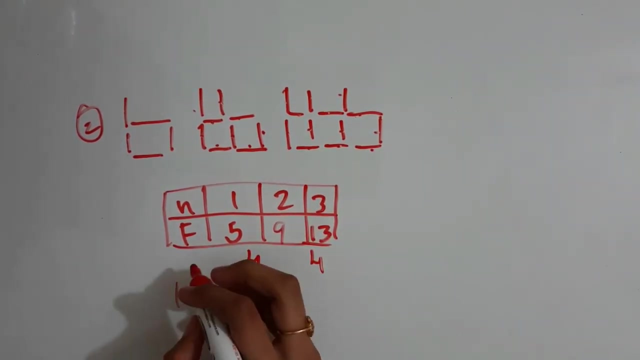 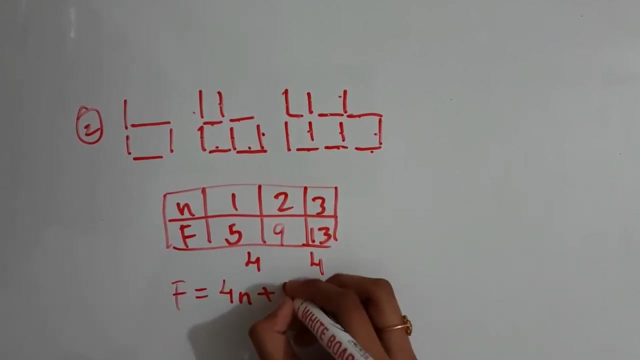 is 5, 6, 7, 8, 9, it increases by 4, and 9, 10, 11, 12, 13, 4. it increases by 4 again. so let's write our formula: F equals 4 in plus 1. so let's check it out for the first figure.